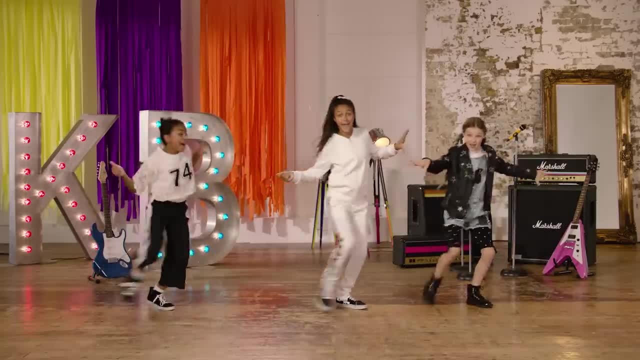 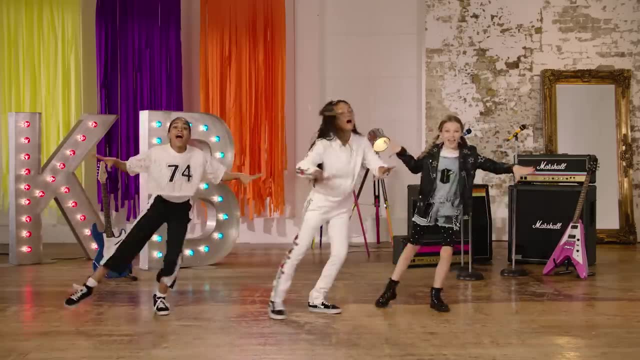 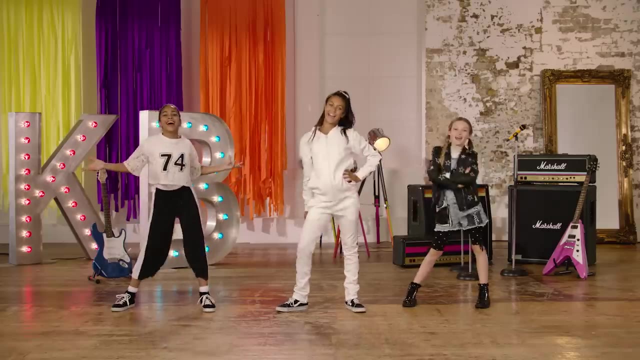 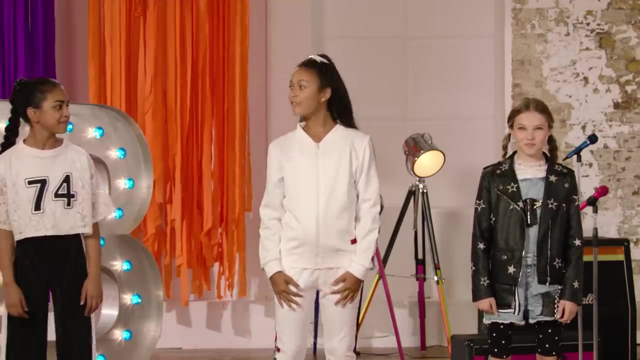 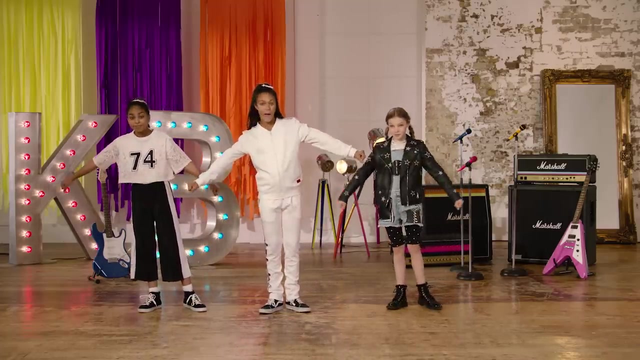 So, guys, we're now going to teach you the steps from Havana. The first move is you're going to get your hand and your arm to the side. then you're going to pull it across, put your both arms out and pop your legs. then you're going to do that to the other. 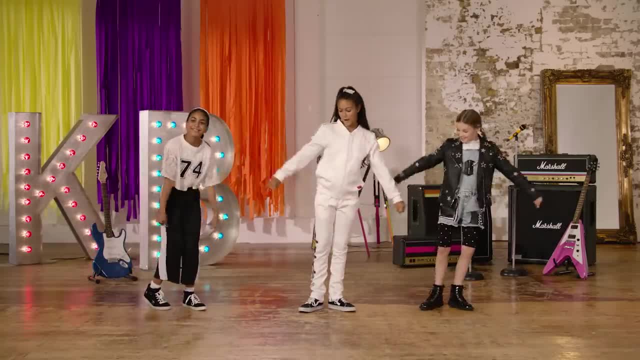 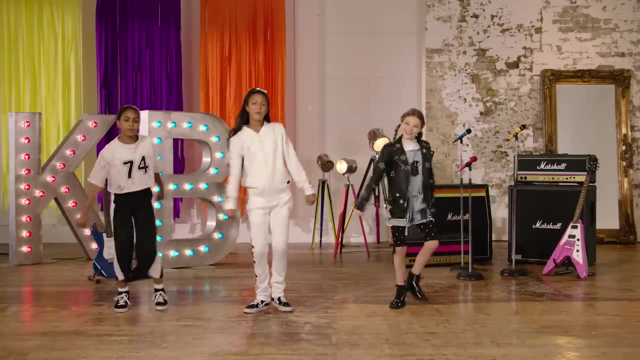 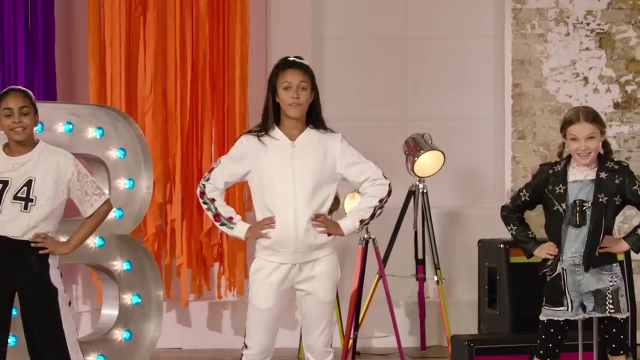 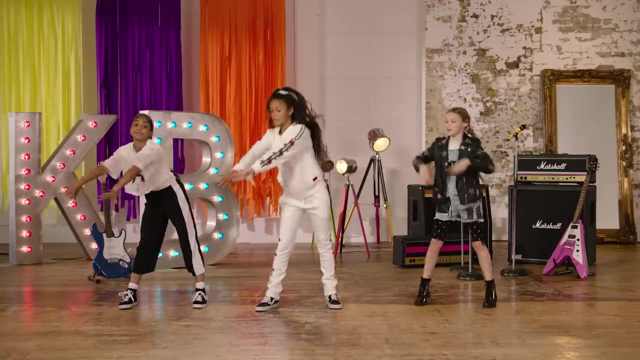 side, arm out, leg out, both arms to the side, pop your legs out, and you're going to do that four times. so you go this way first. I knew it when I met him. so the second move is: you're gonna put your hands out to the side, jump out, and you're going to put them on your hips, so that'll be jump. 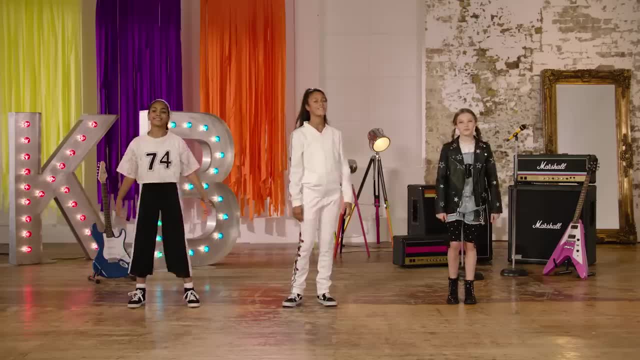 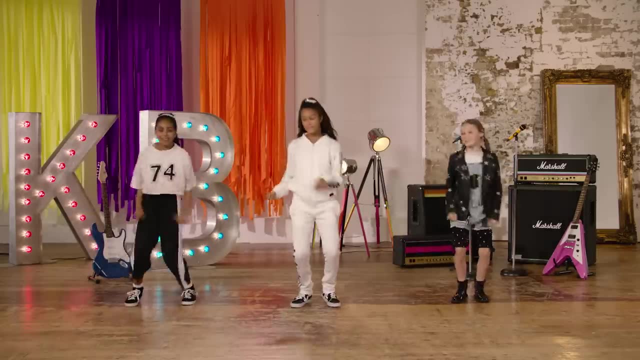 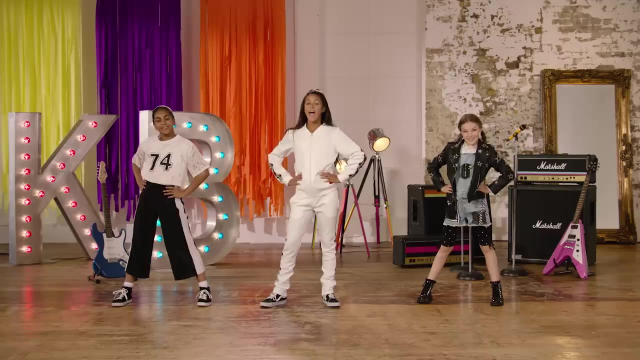 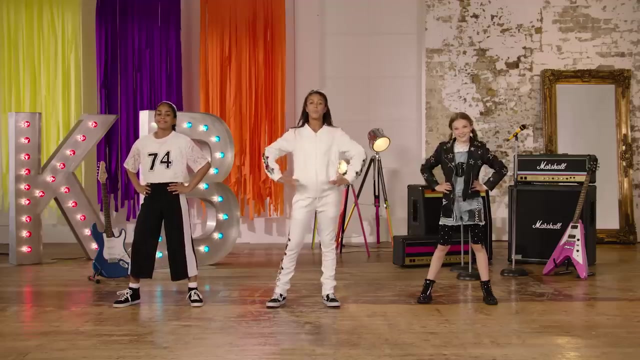 hips ready guys from the top five, six, seven, eight. and then I had to tell them and then it will go. I had to go and then you're just gonna stay there, put your hands on your hips, and then you're gonna put your hands into a fist position by 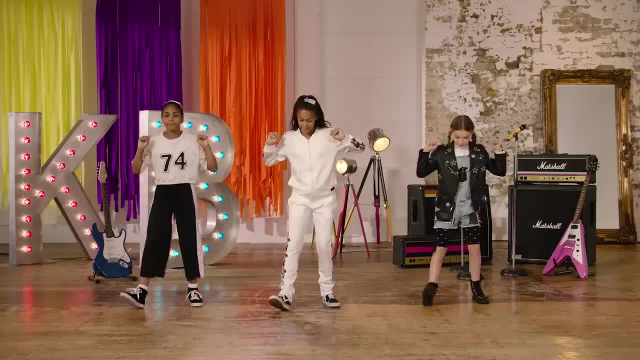 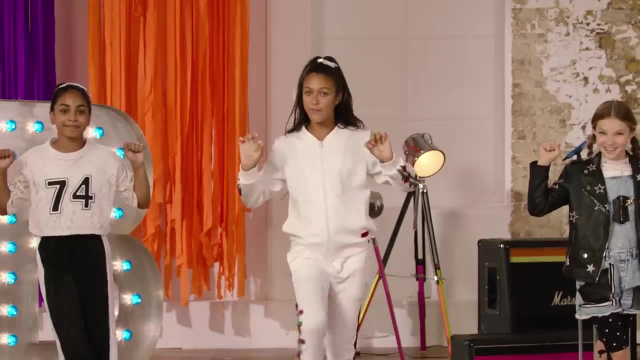 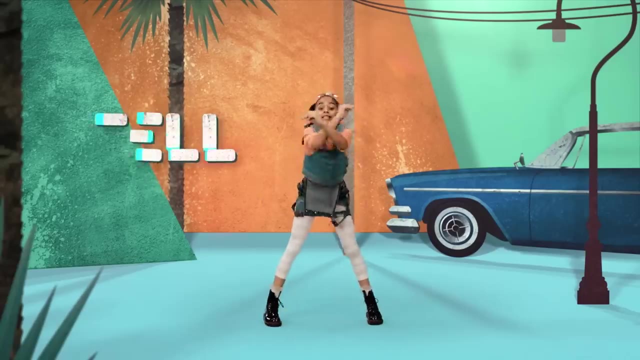 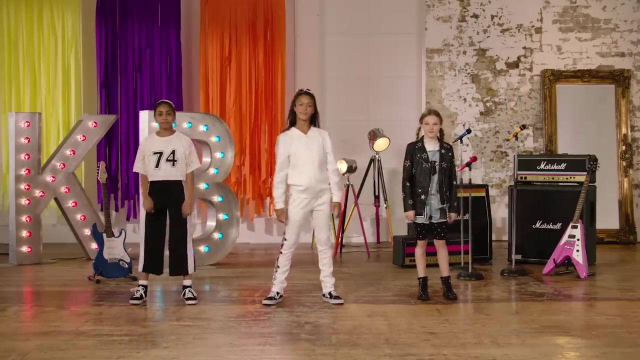 your shoulders and then you'll go heel, heel, toe, toe, heel, and then you're gonna cross your leg with your other leg. so a little bit faster that will go. oh, na, na, na, na na. okay, so gonna go from the top now very slowly. five, six, seven, eight. 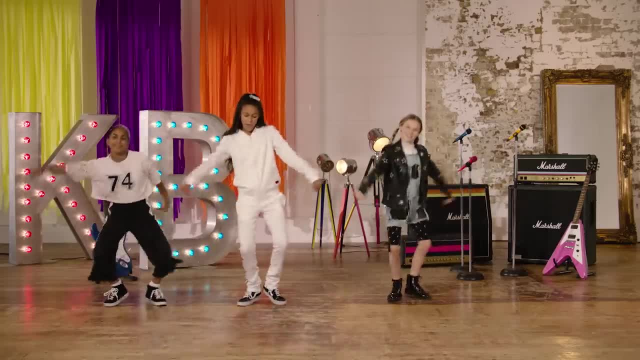 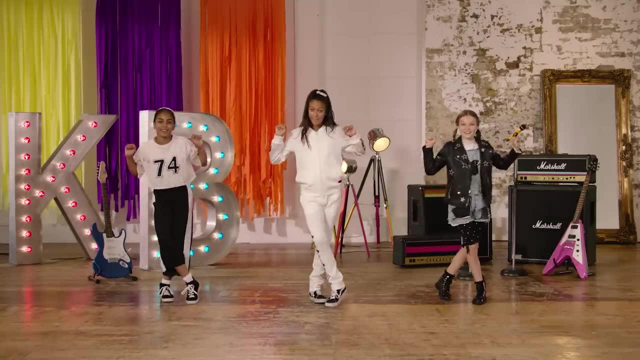 ooooooo, ooooooo, ooooooooo, oooooo, ooooooooooooooo, ooooooooooo, ooooooooooo, oooo, ooooooooooooooo, ooooooooooo, ooooooooooooooooooo. And then I had to tell him I had to go: oh, na, na, na, na na. 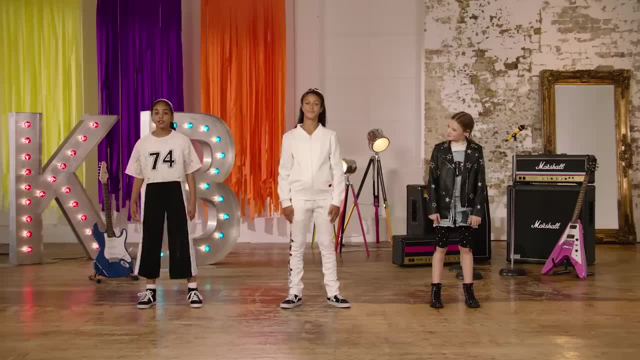 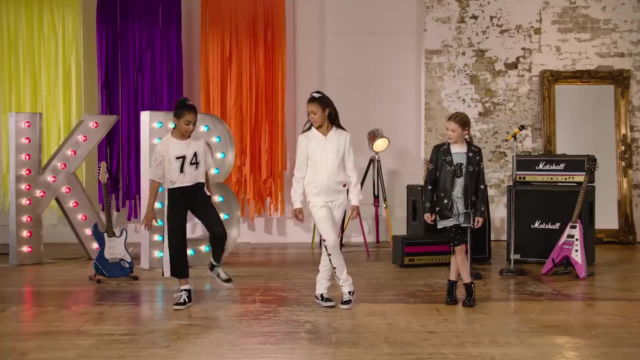 Great job, guys. So now I'm going to pass you over to twinkle. So we've just ended. heel, heel, toe, toe, heel toe. So we've ended in this cross position. So what we're going to do is we're going to step out. 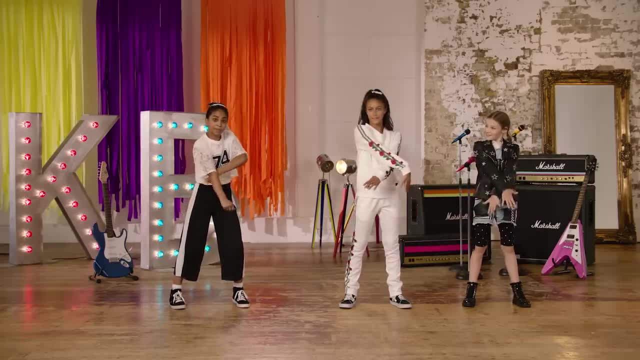 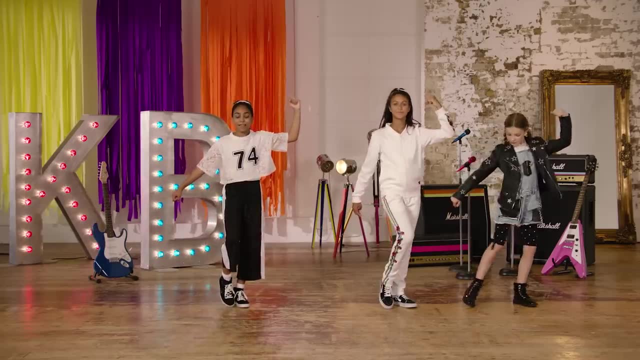 and we're going to cross our hands with it And then we're going to slowly bring them out to this position like this, like we're picking something off the shelf And then we slowly drag this one in And we're going to do the same on the other side. 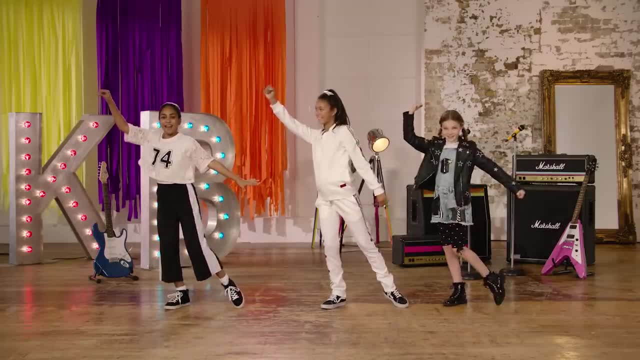 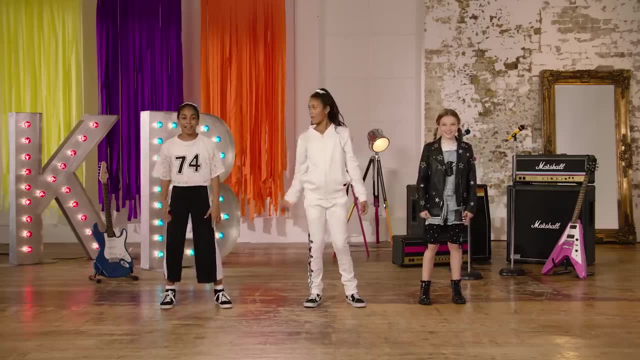 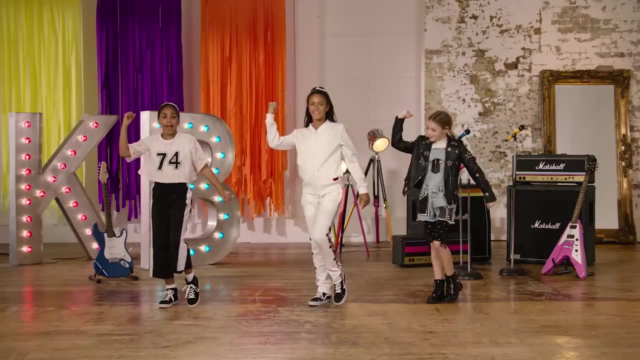 Cross, pick something from the shelf and drag. So you repeat it on both sides. Let's try that. Five, six, seven, eight, Havana oh na na, Havana oh na na. So from here on the hey, we're going. 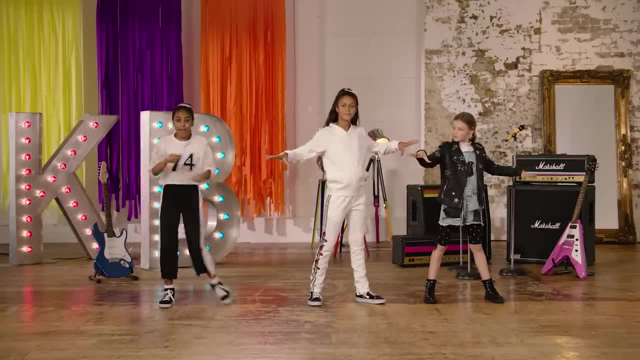 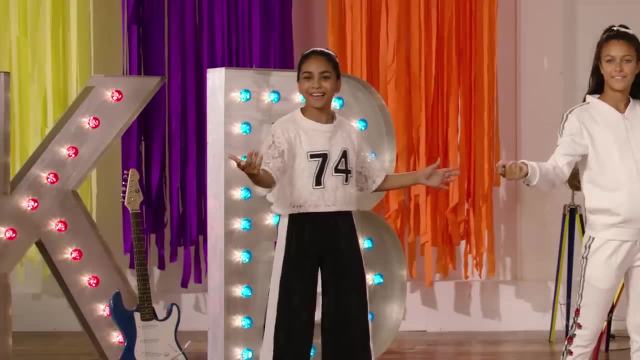 to step out with our legs and our hands like this: Hey, From here we're going to step out, We're going to do a turn and click. It's all right if you can't click, So we're going to roll and click. 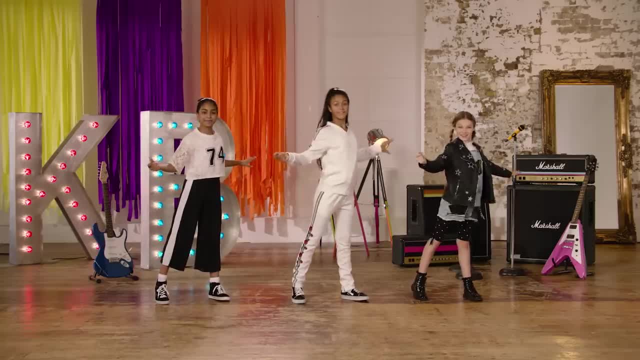 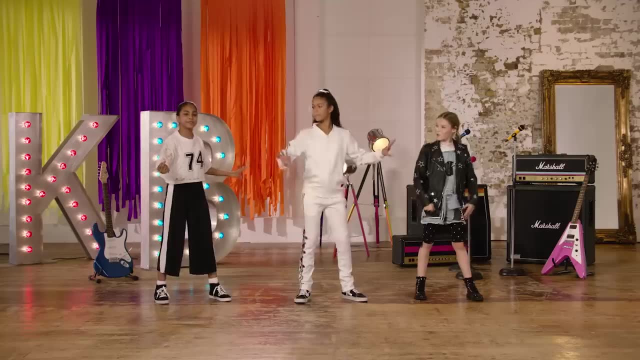 So from here, what we're going to do is we're going to put the chest out, Then we're going to put it in, And then we're going to do a lock in the hips like that. Let's try that move a bit faster. 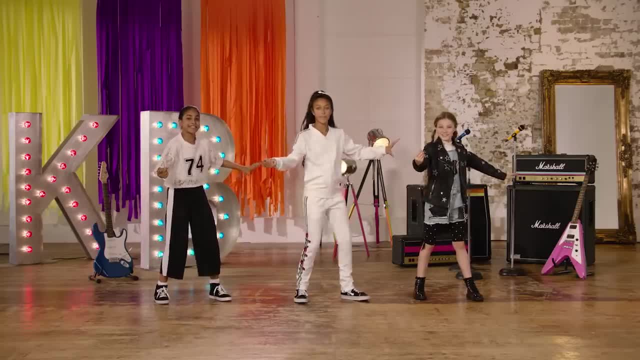 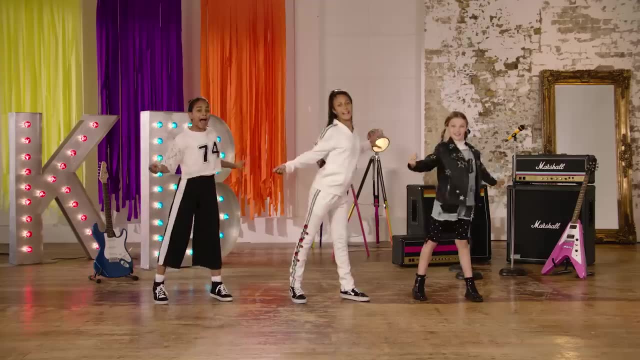 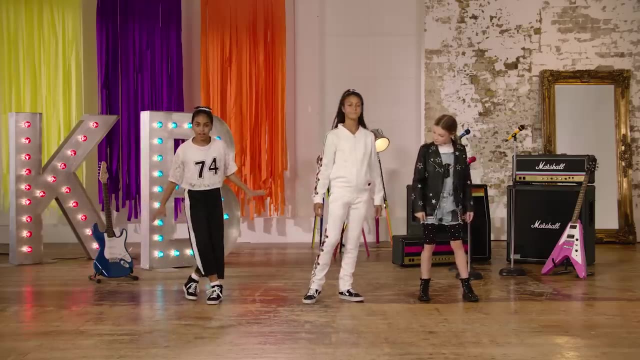 Ready: Five, six, seven, eight Out in drop. And tempo: Five, six, seven, eight Out in drop. Half of my heart is in. From here, your leg is going to come in front of the other. 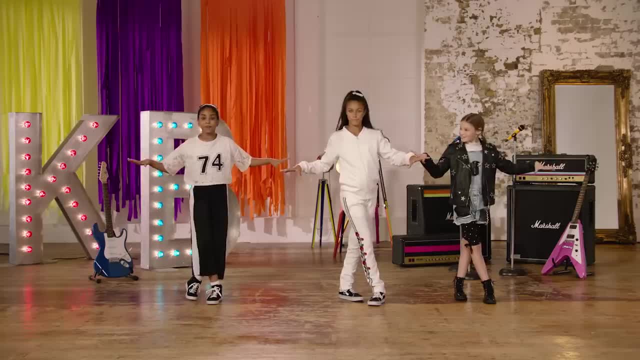 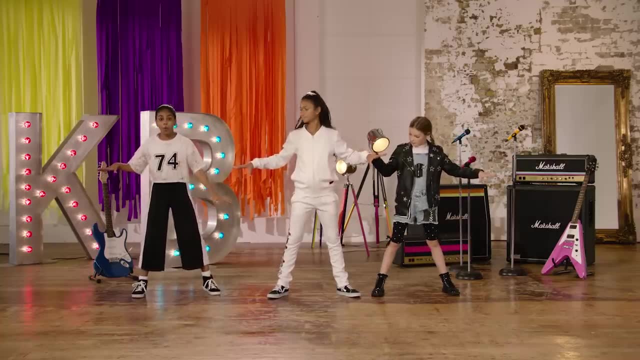 And our hands are going to stay in this position this whole time. So you put it in front, Then we're going to step behind, Then we're going to step to the side And then all our weight goes onto this leg while we pick this up into a 90-degree angle. 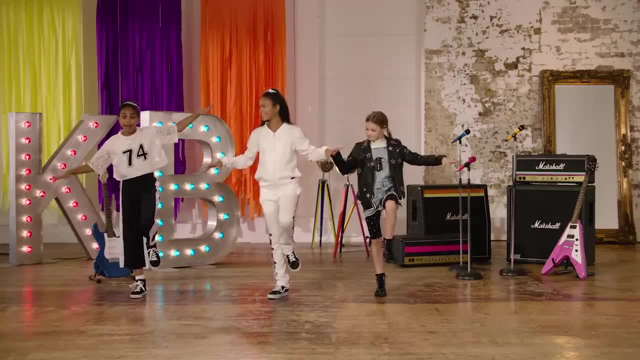 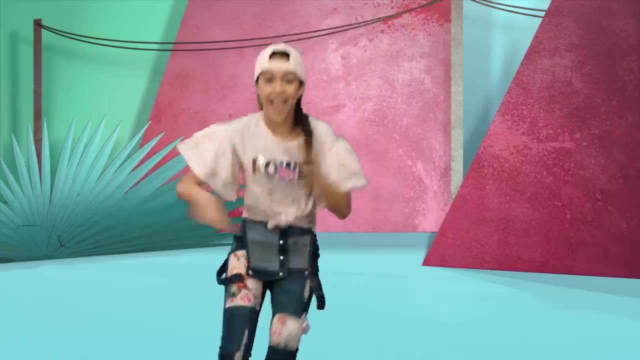 Perfect. So from here, what we're going to do is we're going to do a big slide out to this side And while we do that, you're going to make sure you have this position In Havana, ooh, Havana, ooh na na hey. 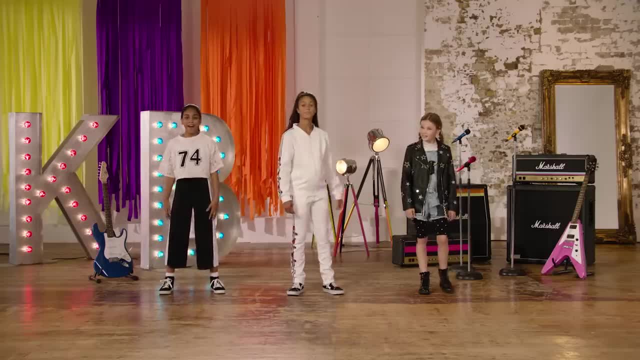 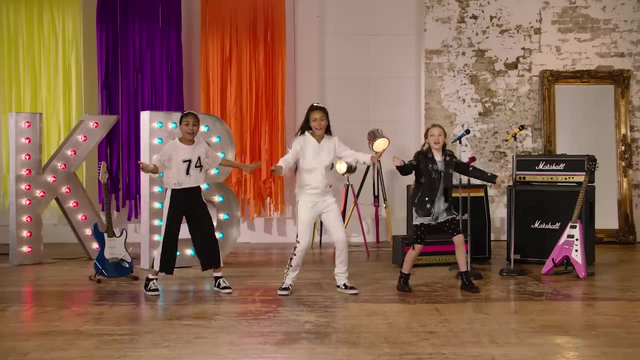 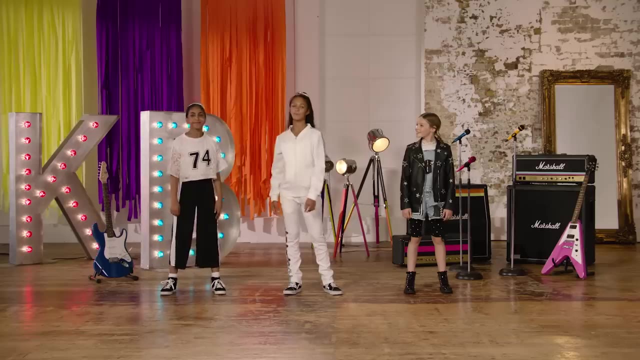 So let's do this whole section together. Ready, Yeah. Five, six, seven, eight. Havana, ooh na na hey. Half of my heart is in Havana, ooh na na hey. Now we're going to do it from the very, very top. 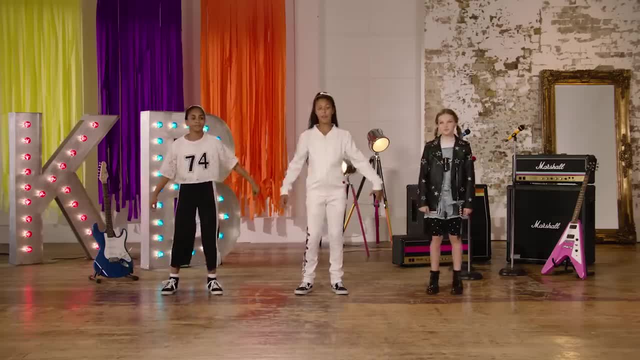 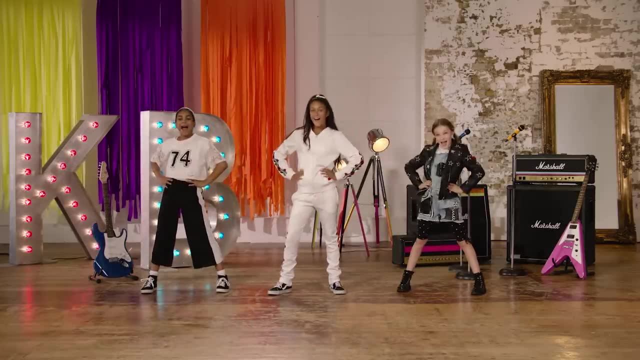 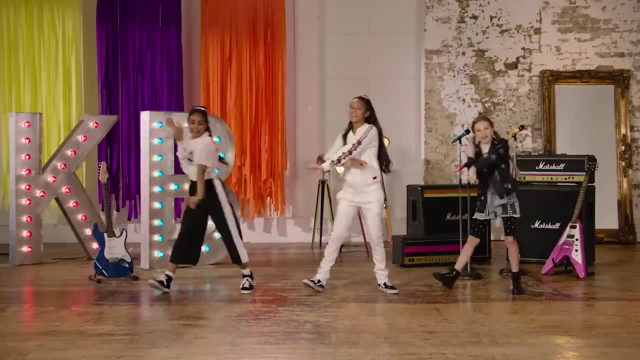 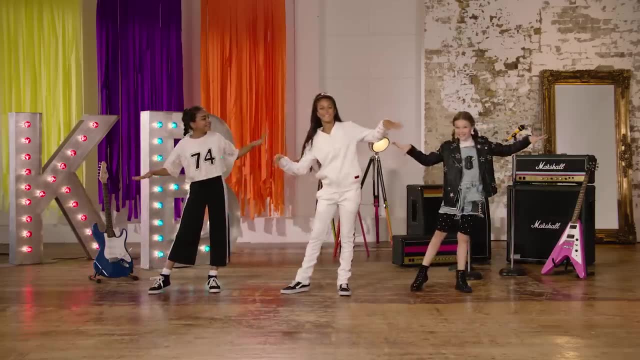 Oh na na na na na, Havana, ooh na na hey. Half of my heart is in Havana. ooh na na hey. So now Mia is going to teach the next bit. 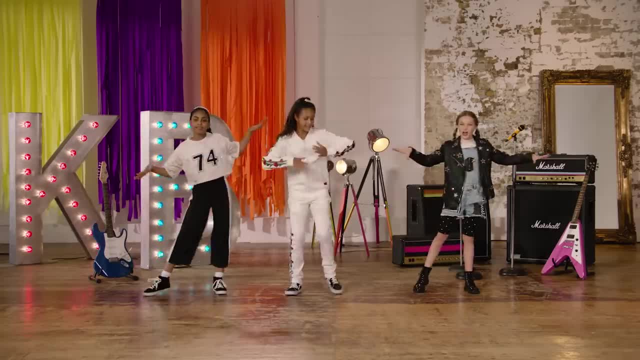 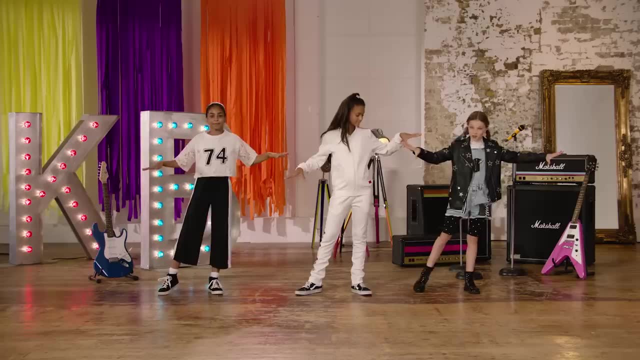 Thank you, Right, so we've just finished with a slide on hey, And that's on count one. Now what we do is we have all of our weight on this leg, So with the leg we have free, which is this leg, 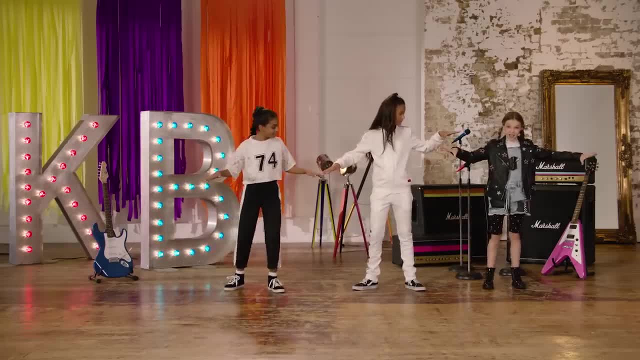 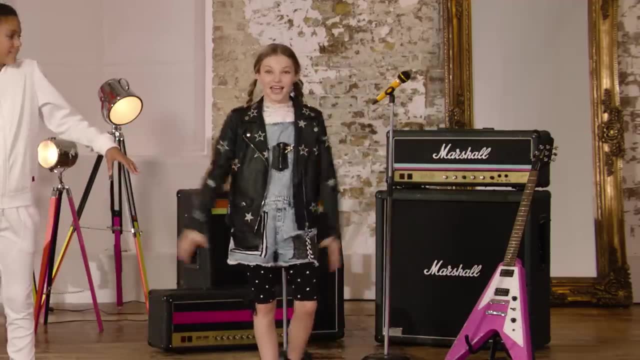 we step it behind, And then to the side, And then to the front, And once you do that, every time your foot goes down this shoulder pops up. OK, so let's try that now. Five, six, seven, eight, one. 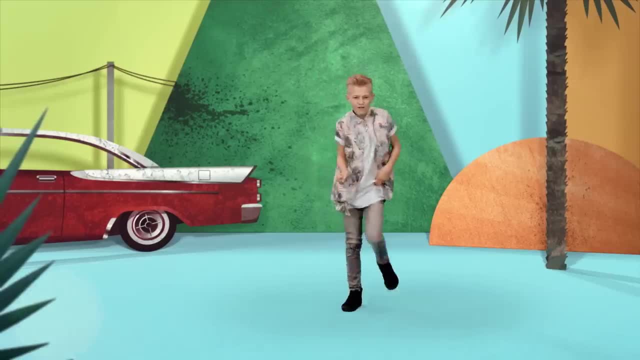 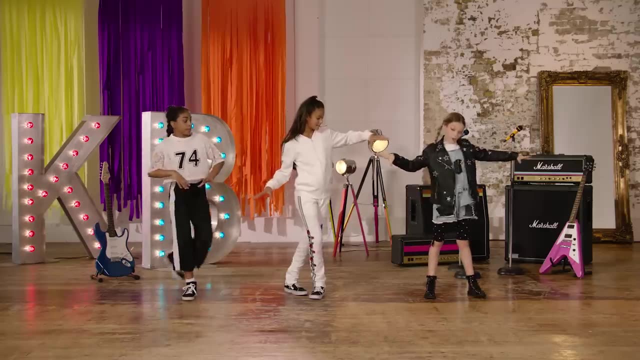 It took me back to east. It took me back to east. The next thing we do is, because we have all of our weight on this leg, we take the one from behind and pop it to the side, whilst our arms swim through and end up at the back. 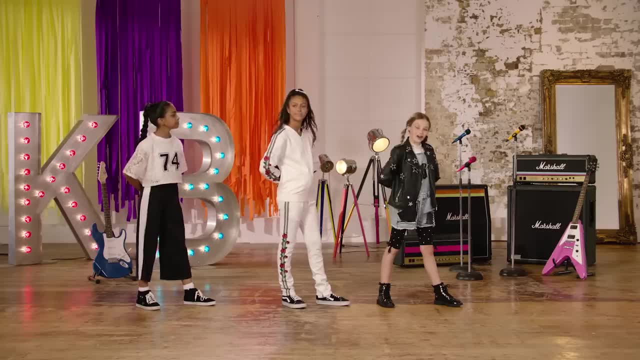 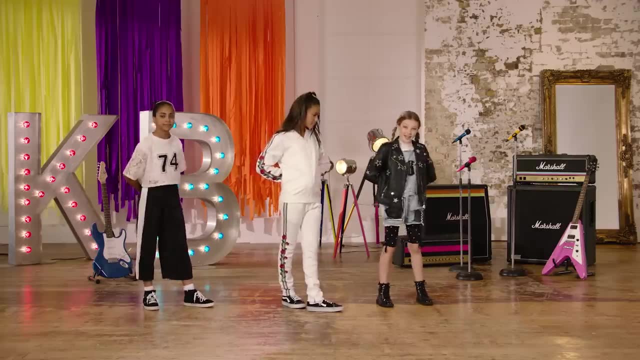 Whilst our head is looking at our foot, And that's on Havana. Then our head goes down on Atlanta, And then we do a heel, toe, heel on na na na, East Atlanta, na na na. So let's do that from the top. 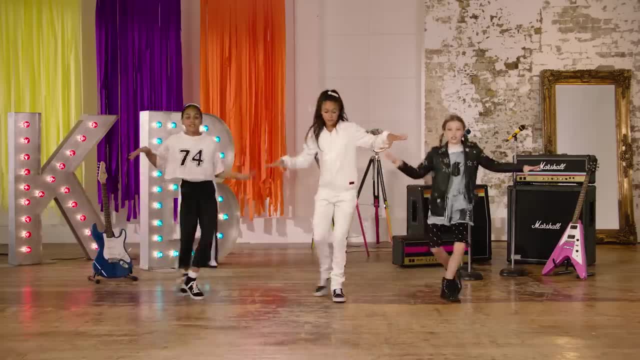 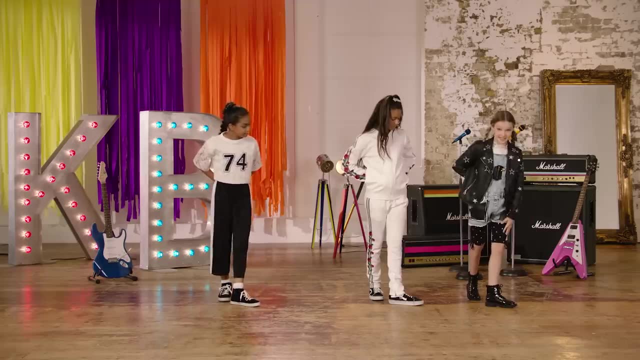 Five, six, seven, eight, one. It took me back to east Atlanta. na na na. OK, so now we have all of our weight on this leg, So we're going to put this one to the side And then this leg comes up into a 90.. 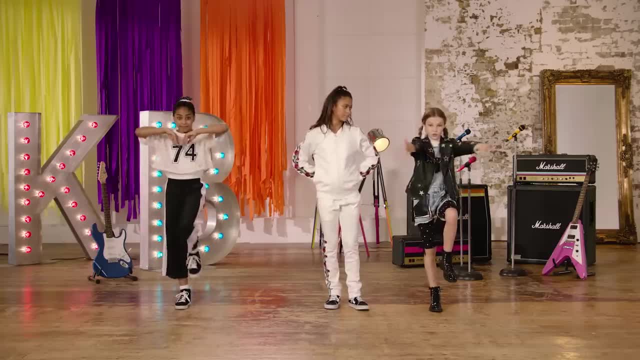 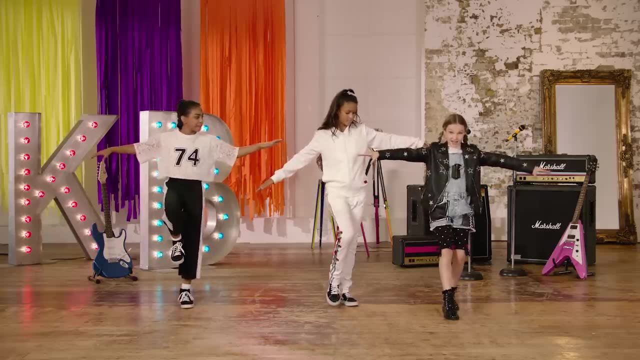 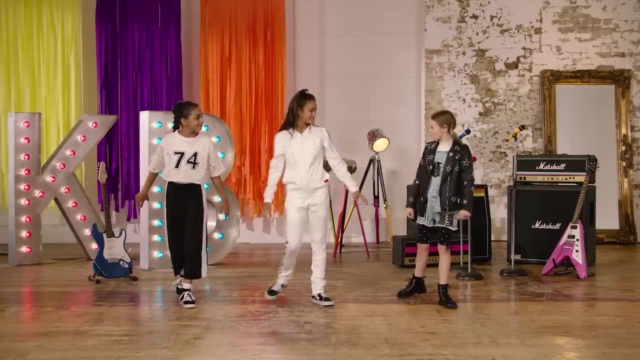 90-degree angle And our arms swim out and stay to the side of us, And then we jump onto this leg And this stays on the floor And our toes swims out with our arms as well. OK, so you do that from the top of my section, really. 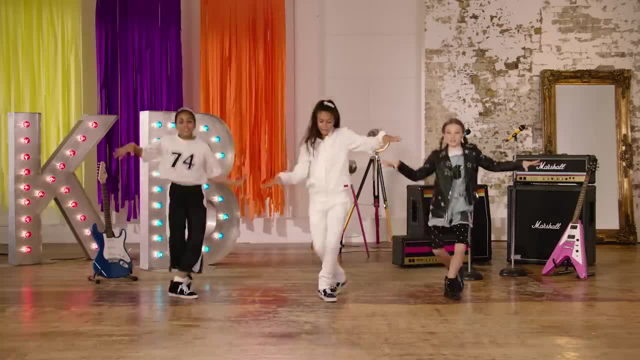 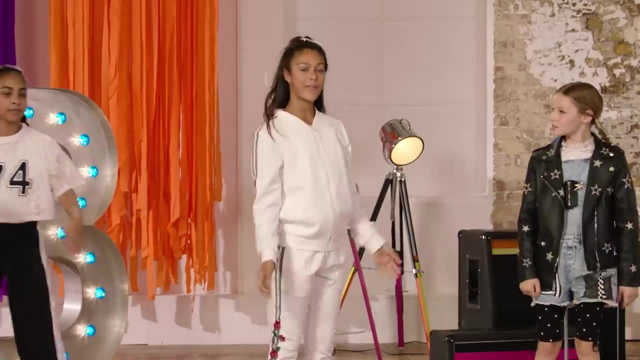 Five, six, seven, eight one. It took me back to east Atlanta. na na, na, Hey, And then we've just ended up from the hey And we're going to put our leg behind the other leg And then we're going to step it out. 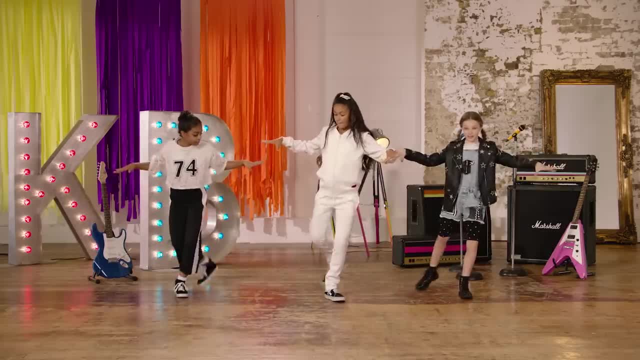 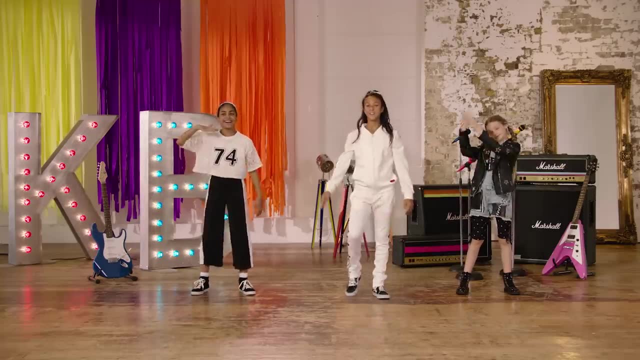 But you're still in this position, So we'll go hey back and then side, And then you're going to imagine you have a beach ball right here And then you're going to put your arm over it while you step your leg out. 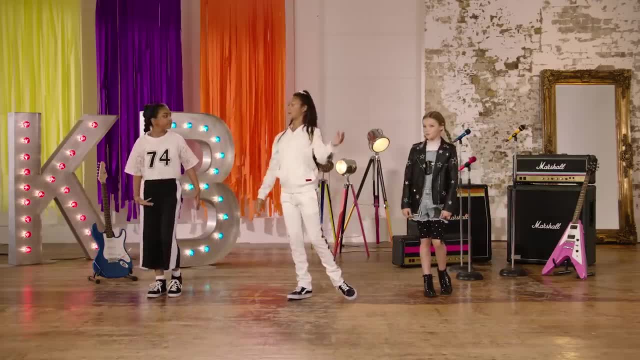 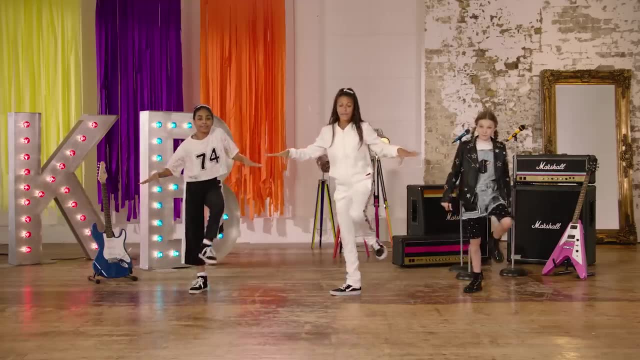 So you're going to go step And then you're going to do that same on the other side: Step. So from the beginning that will go: hey, Step, Step, Step, Over Over. So we're going to do that a little bit quicker. 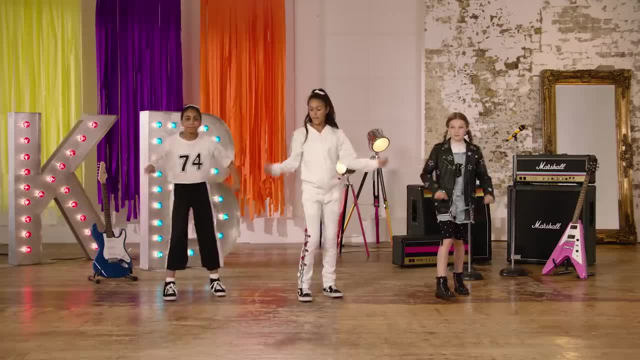 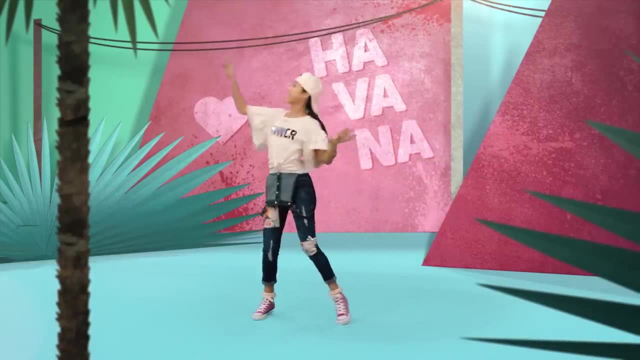 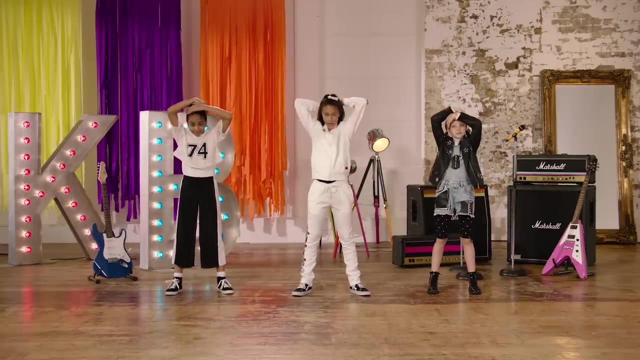 Ready: Five, six, seven, eight, Step, Step Over Over, And then we're going to cross our arms like this And we're going to put them behind our head around onto our shoulders And then bring them across your chest and out. 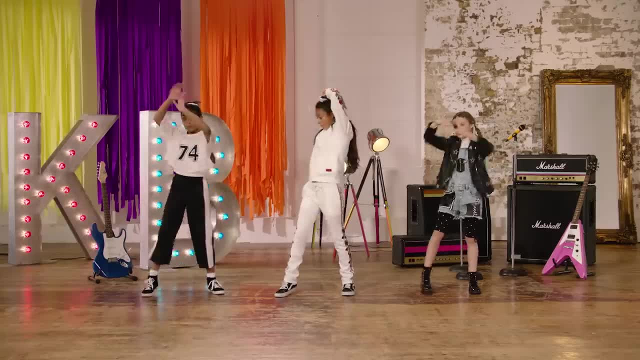 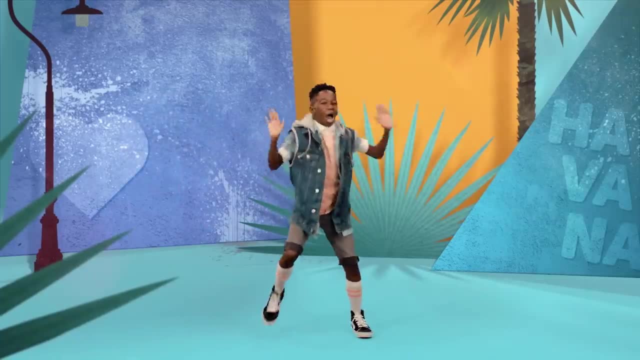 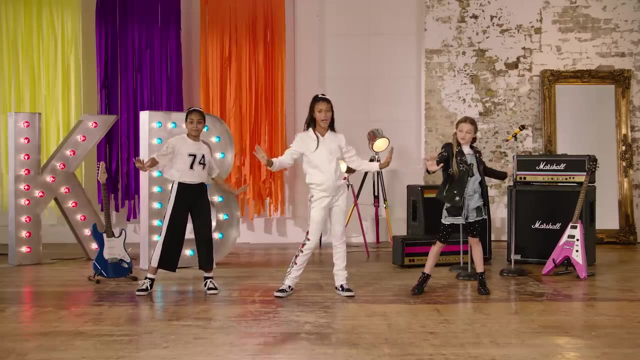 While you're stepping your leg, this leg first. you're going to go round shoulders, through your chest and out. My heart is in Havana, And then we'll go with this hand. first, We're going to go round round. 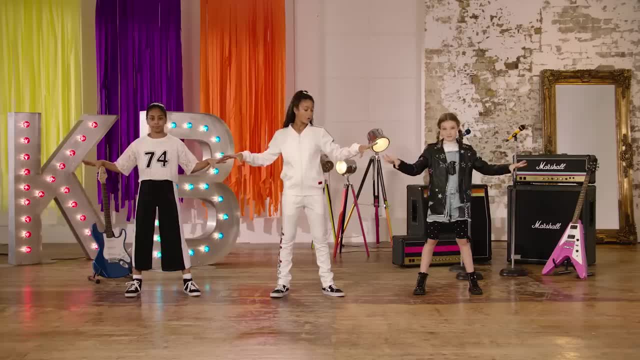 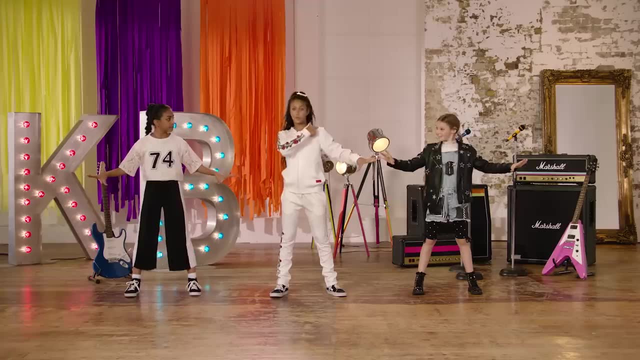 At this part, you're going to put your hands like this: You're going to control your knee with your hand And you're going to go up and up, Up, Up, Up and over, Up Over, And you're also going to roll your shoulders back. 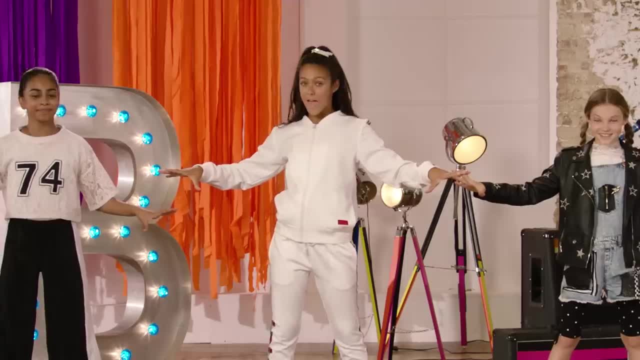 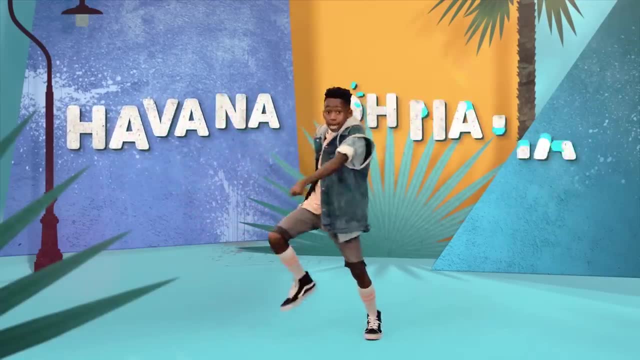 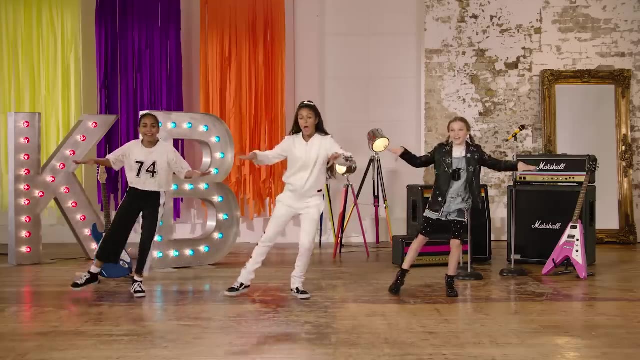 Up and over, Up and over, And then you're going to do whatever pose you want: Five, six, seven, eight Pose: Havana, Havana, ooh, nah, nah. So from the beginning of this section it will go five, six, seven, eight. 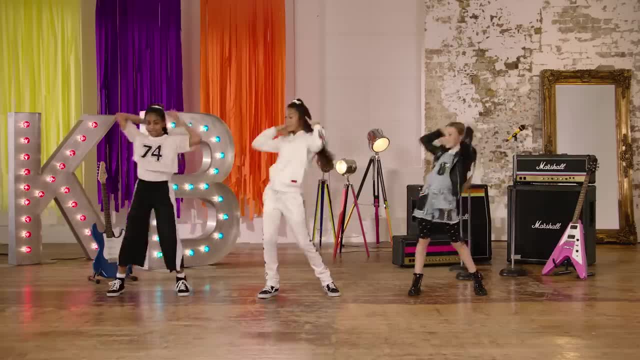 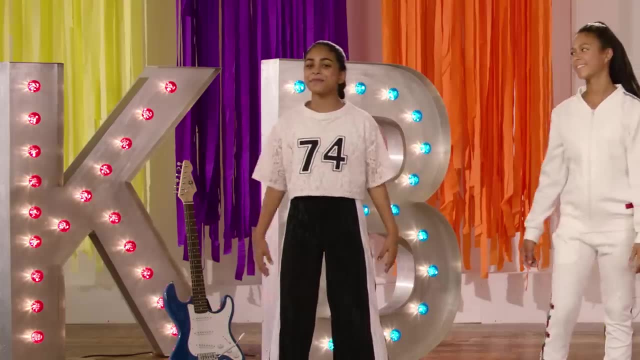 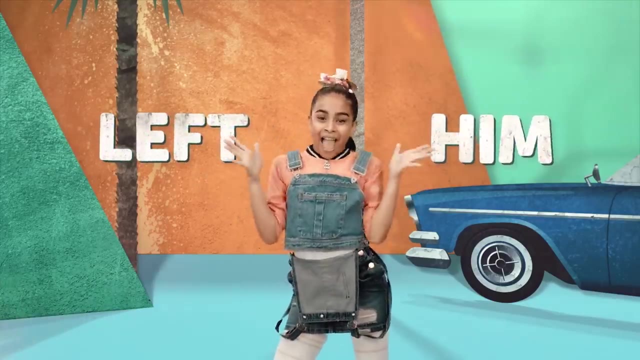 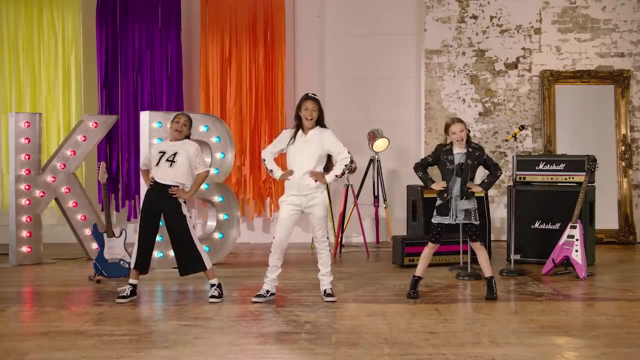 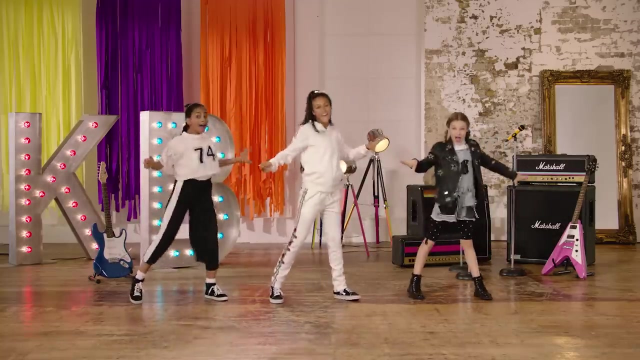 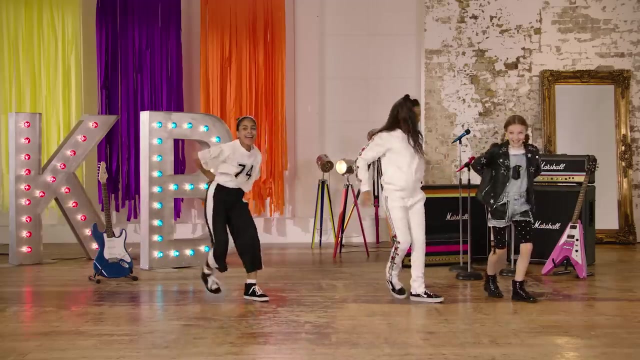 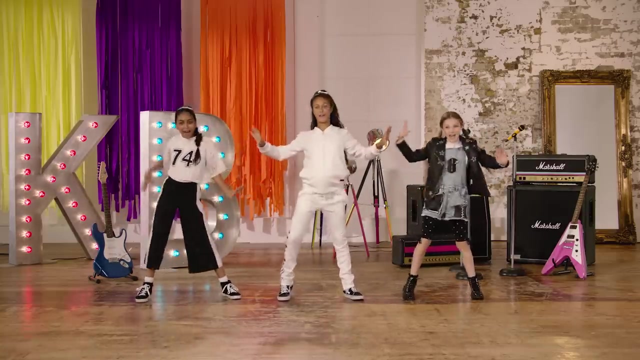 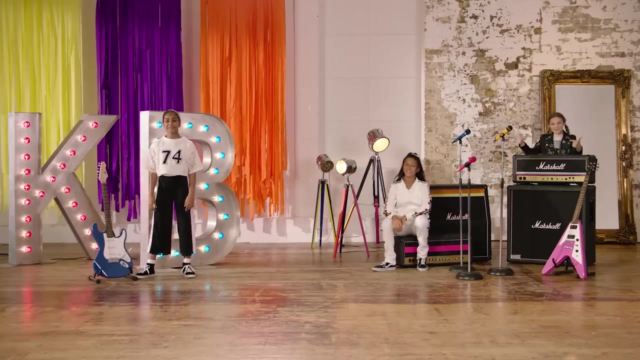 All of my heart is in Havana. There's something that is manners. Havana, ooh, nah, nah. Well done everybody. Now I think we're ready for the moves and music. That was awesome. everyone, Good job. Don't forget to hit the like button and leave a comment below. Bye, Bye.